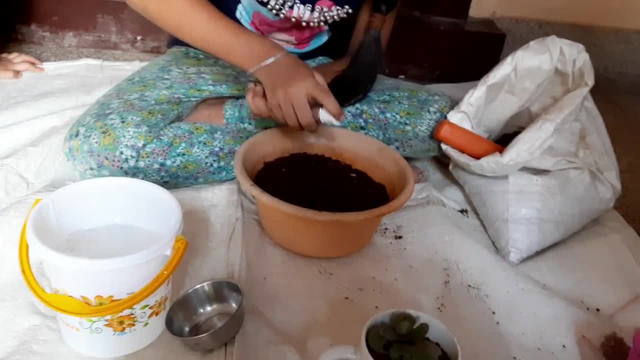 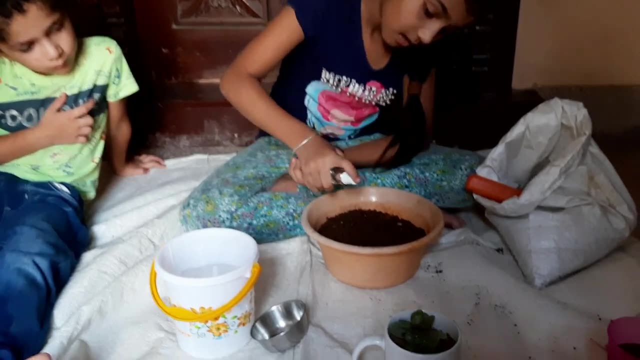 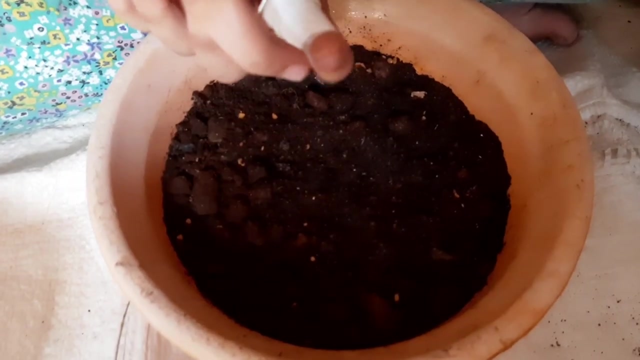 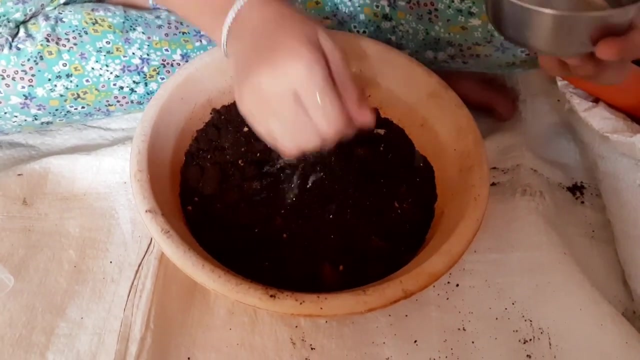 Sprinkle water: 160.. Yes, 50,000.. Uh-Huh, hold on, Hold it quickly. Keep it a little bit near the wheel, Slide down. Good job, See. you see the soil Walk through it. 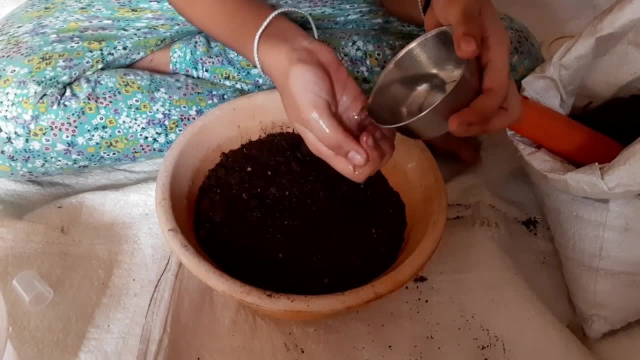 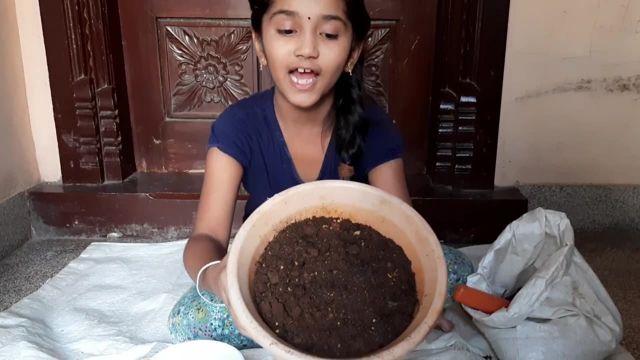 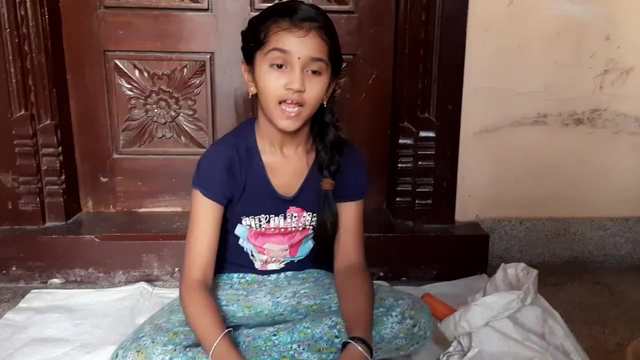 Then you water again, Stir, well, Okay, 1,, 2,, 3.. Now, in 2-3 days, the methi plants will grow nicely. My mom used this cup for plants. See how it is nice. no, Now let's check the coco peat is ready or not. 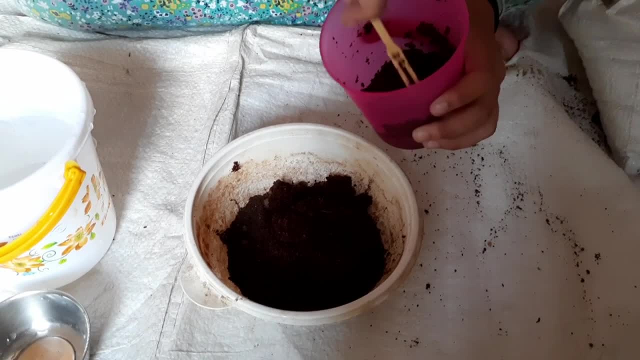 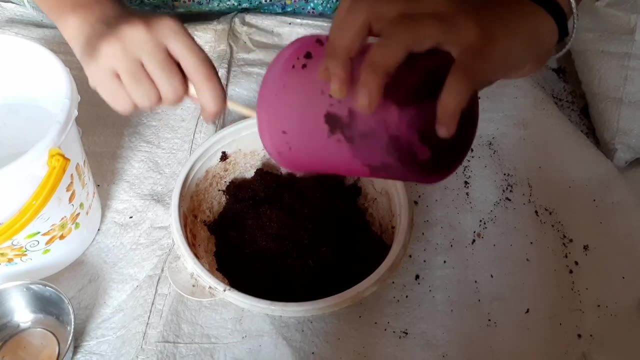 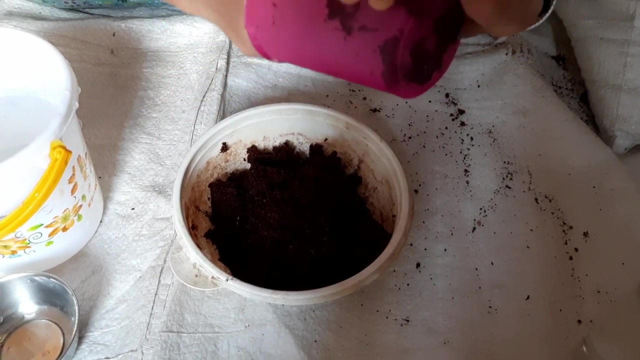 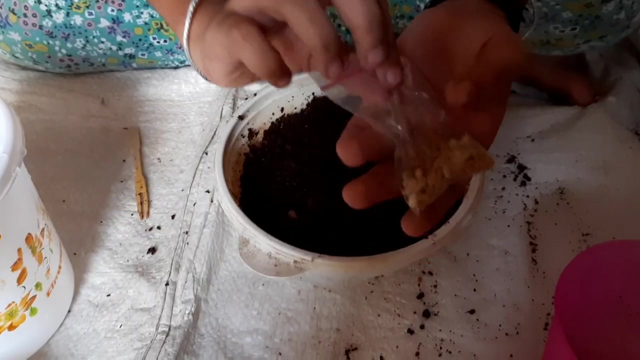 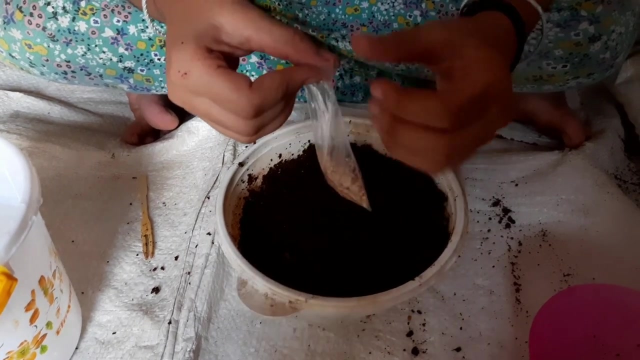 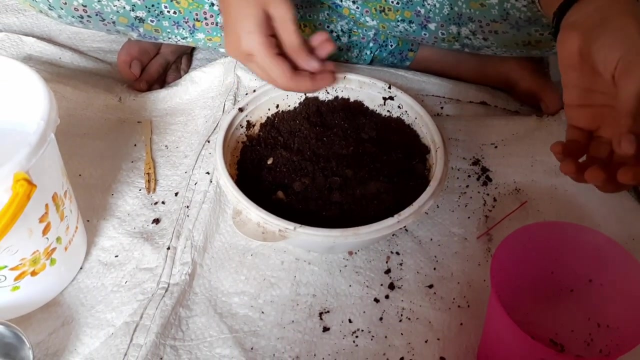 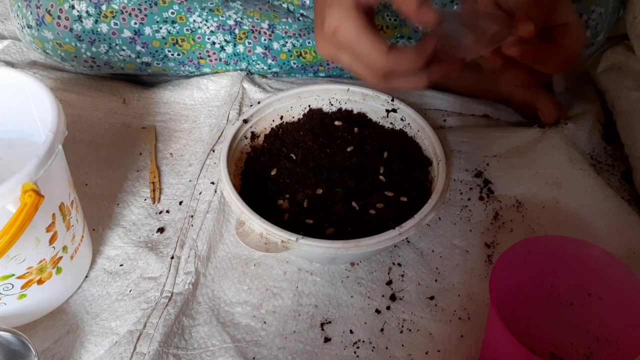 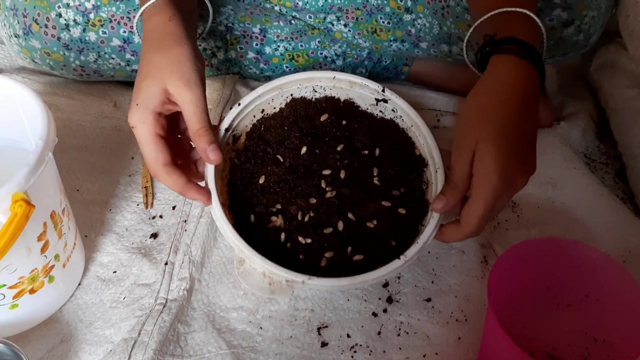 The coco peat is ready so I am adding into the container. We got wheat seeds in kit itself. We can use it In the same way: take little bit and sprinkle it. So after sprinkling it we can add soil Very little. 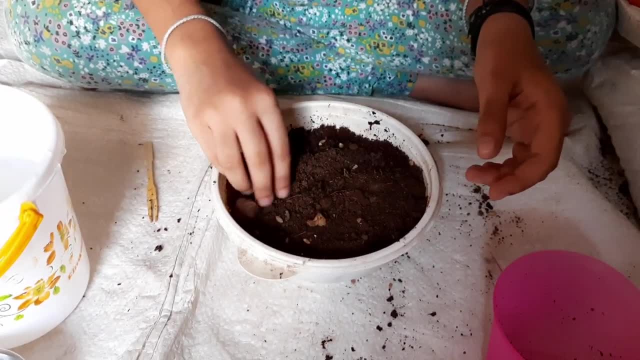 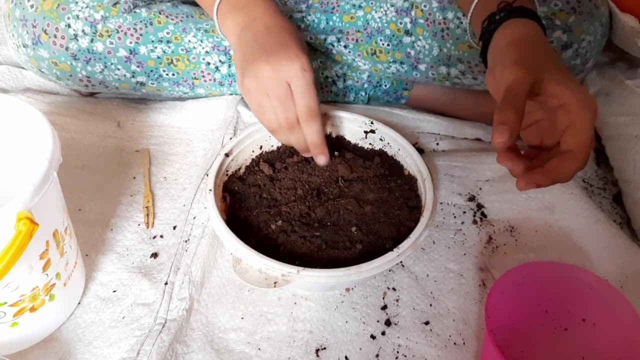 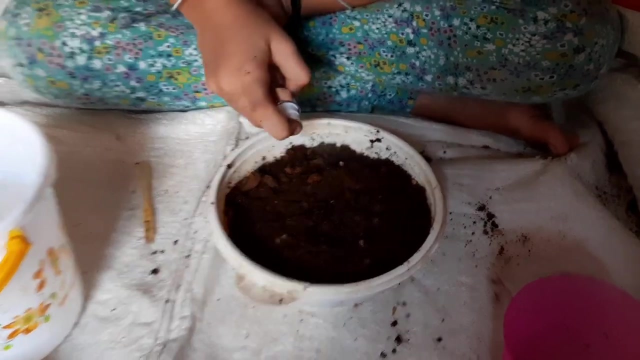 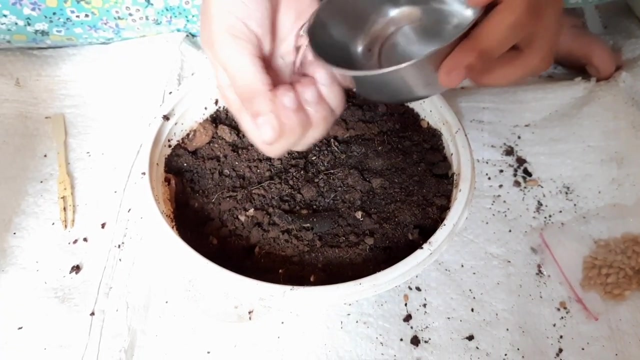 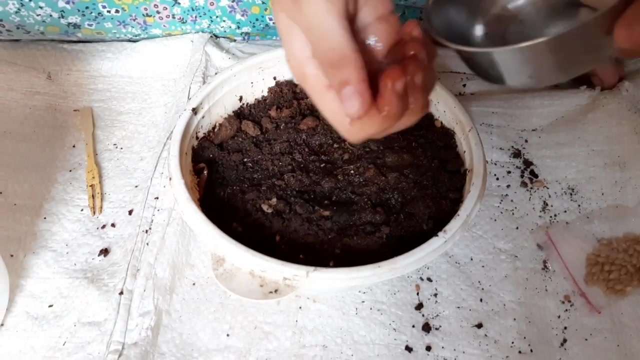 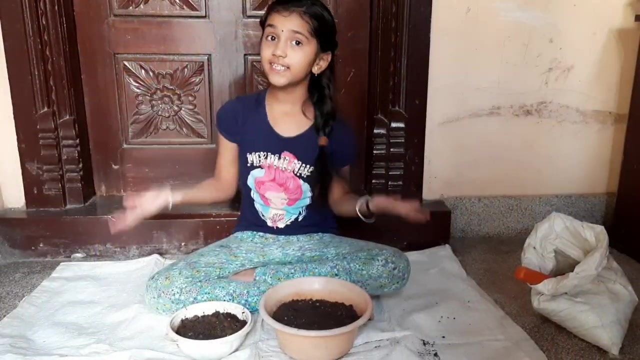 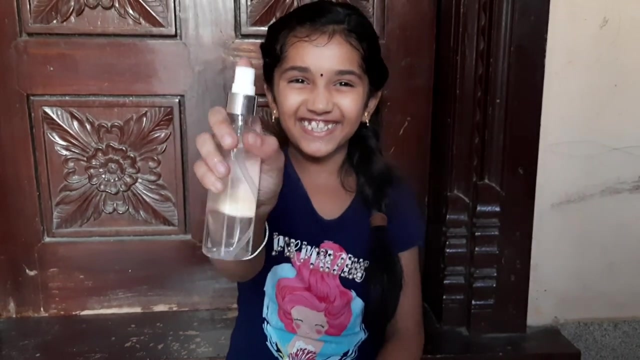 Enough. Okay, So we can add And water little bit in this. So enough, That's all We have done. 2 plants In today. I really like this Push, push There. See, Jolly See.